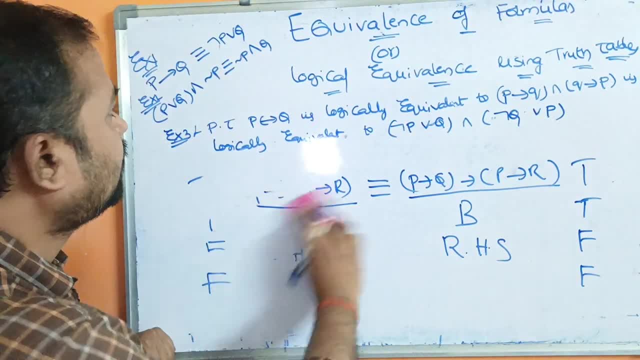 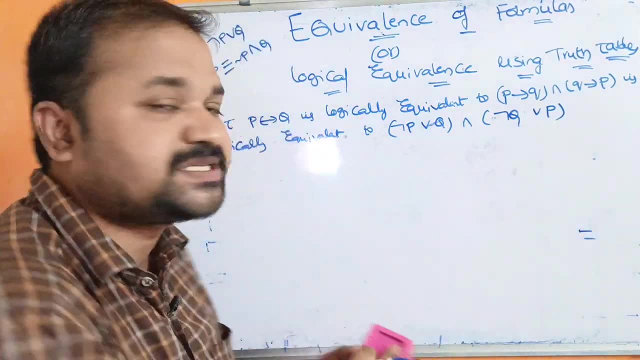 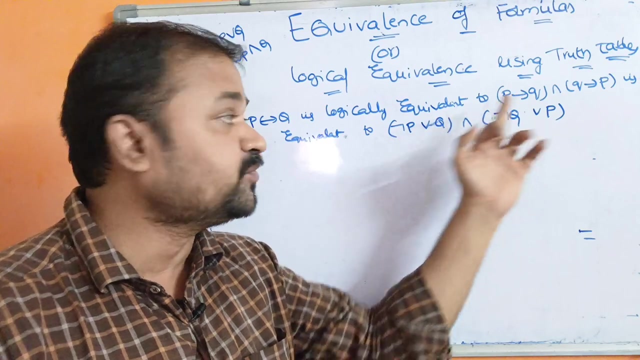 equal. So this is the. this is about what is equivalence of formulas. So when we can say two prepositions are equivalent, this formula means statement formula. Here, this is a statement formula, negation PRQ. This is a statement formula or logical equivalence using truth tables. 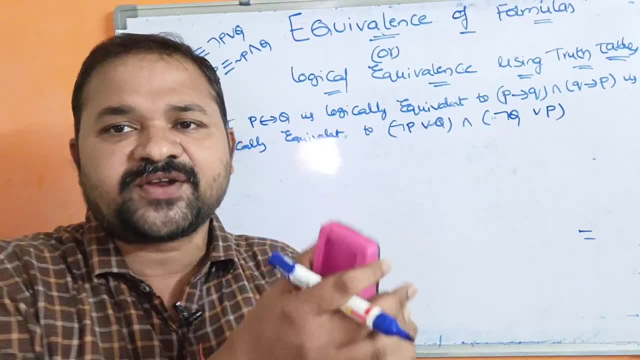 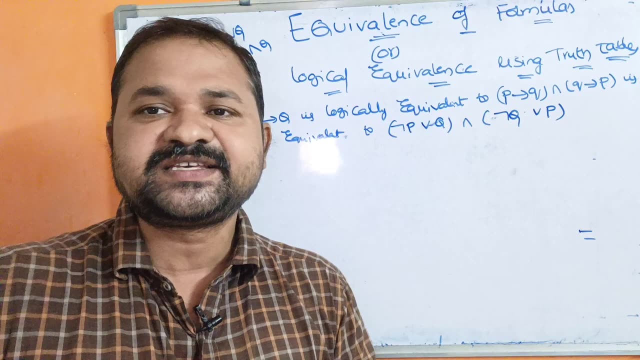 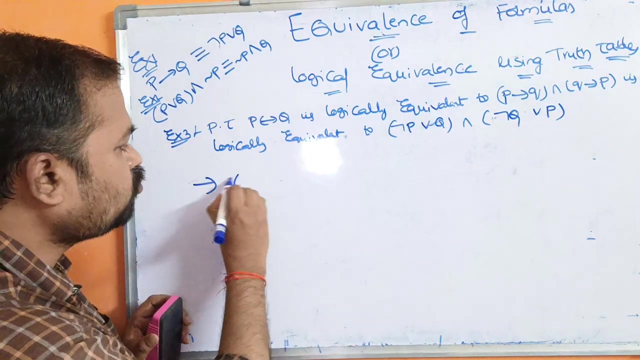 Here we can prove whether two prepositions are equal or not using the truth table as well, as we have one more approach is there, using inference rules that we will see in the upcoming videos. So here the point is: two prepositions, two prepositions. 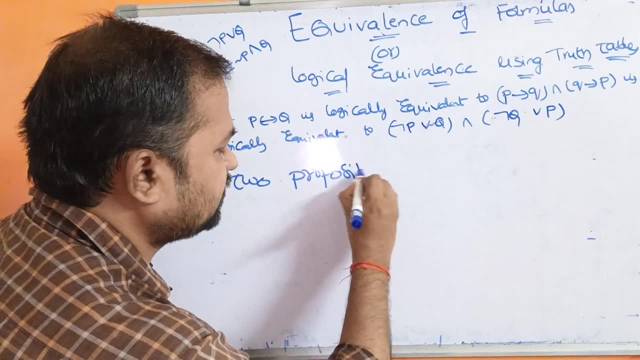 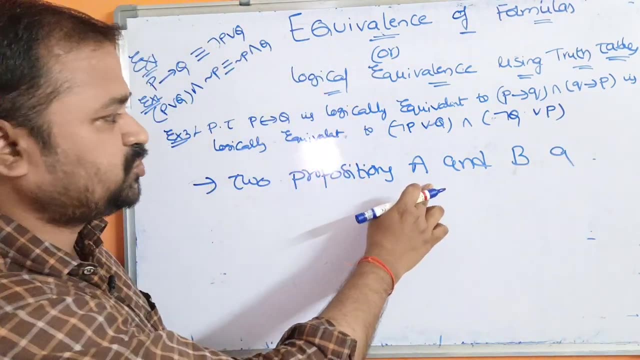 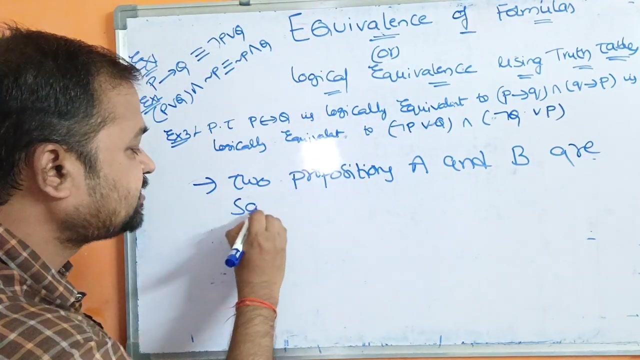 two prepositions, A and B, are A and B are here. A means some compound preposition. Why? Because it contains some correctives also. Okay, Two prepositions, A and B, are said to be, are said to be logically. 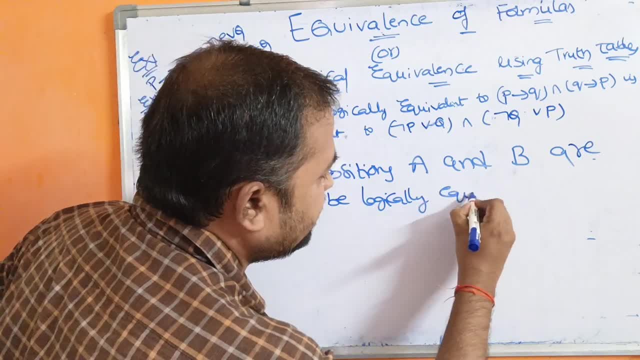 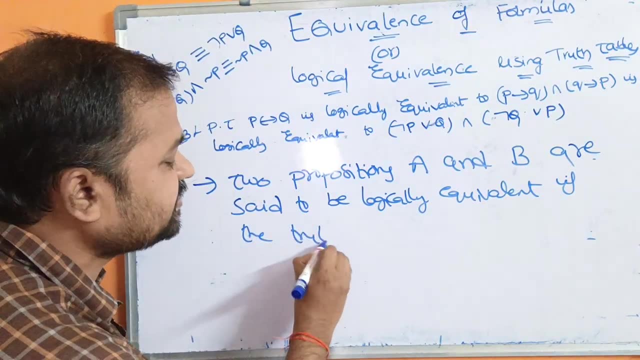 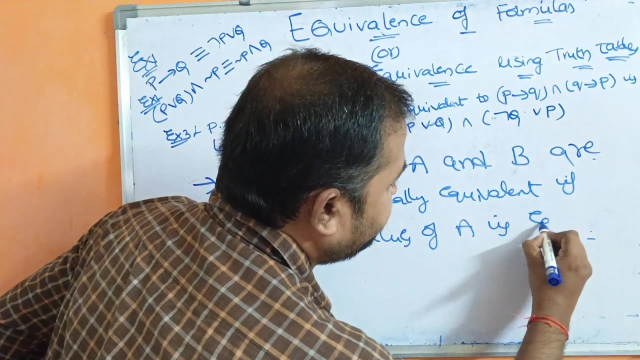 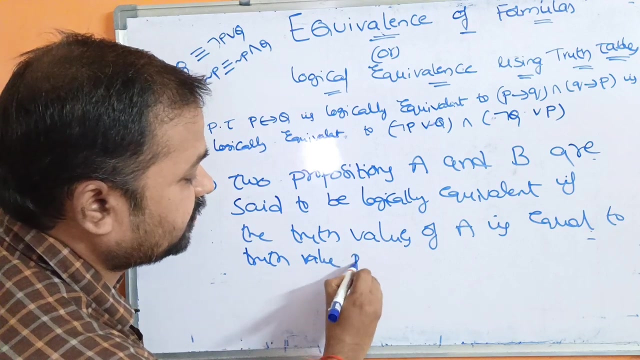 equivalent are said to be logically equivalent. if, if the truth values- So truth value means A is, it may be either true or false. If the truth values of A is, if the truth values of A is equal to, equal to truth value of B, truth value of B for all possible 2 power. 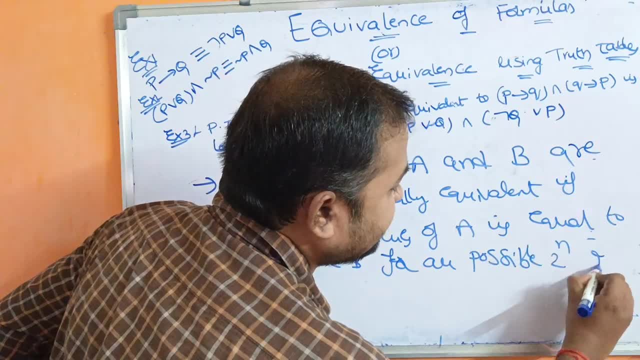 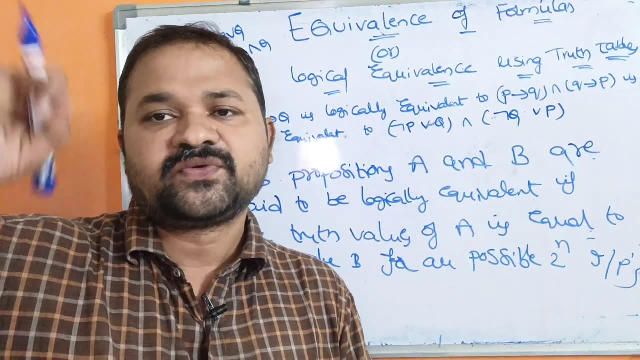 n inputs for all possible 2 power n inputs. So if we consider this problem here we have two prepositions. are there? So 2 power 2.. Slide 39.. 년 2月19.23, lunch 속 censor meeting io2colon&Cow chegou. 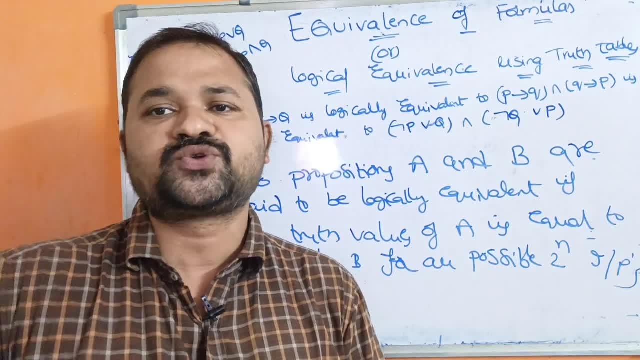 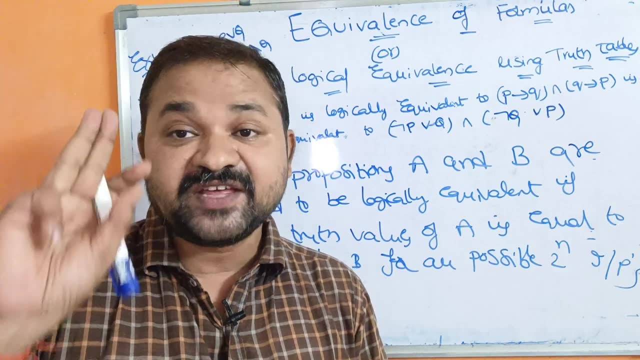 possible combinations are four: True, true, true, false, false, true, false, false. If we have only one proposition, then the possible combination is 2 power 1,. two combinations If there are three inputs: P, Q, R. if there are three propositions, then the possible combinations are 2 power 3,. 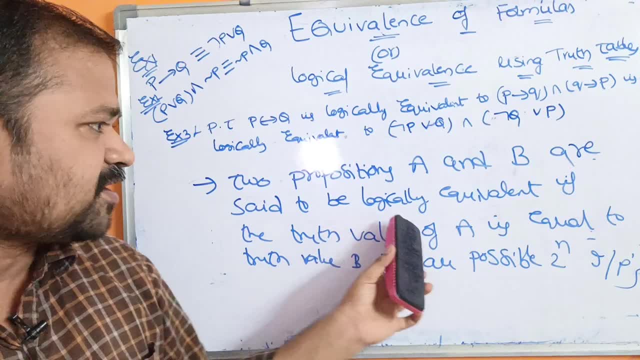 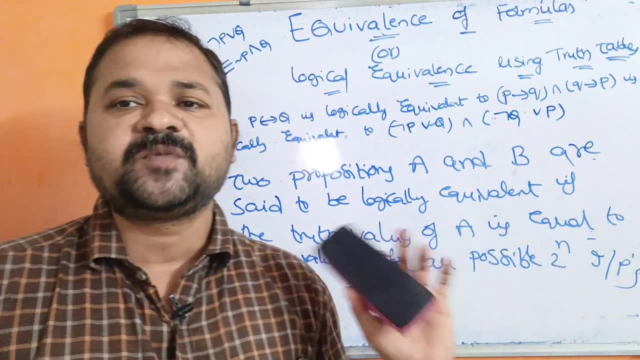 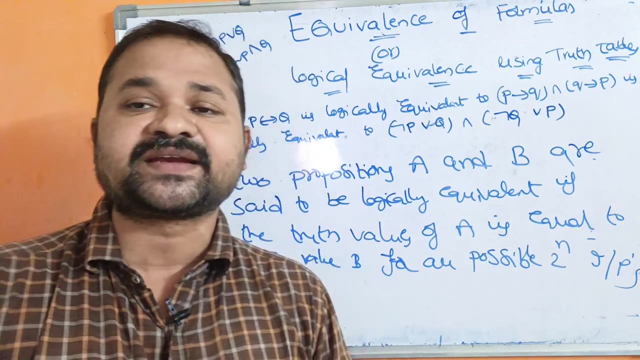 that is 8.. So two propositions, A and B, are said to be logically equivalent If the truth values of A is equal to truth values of B for all the possible two power inputs. So that means we can say that two propositions are logically equivalent if the final columns in the truth 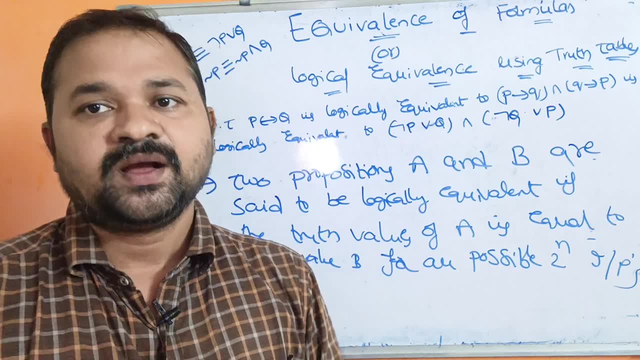 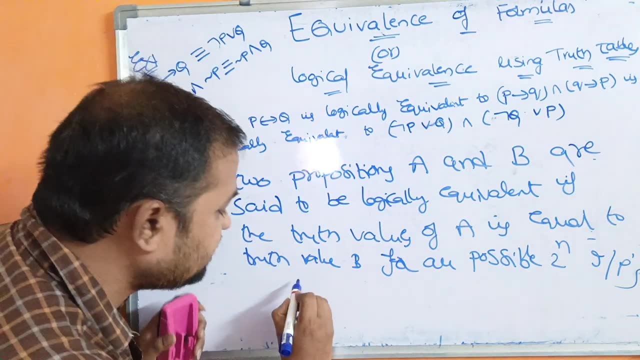 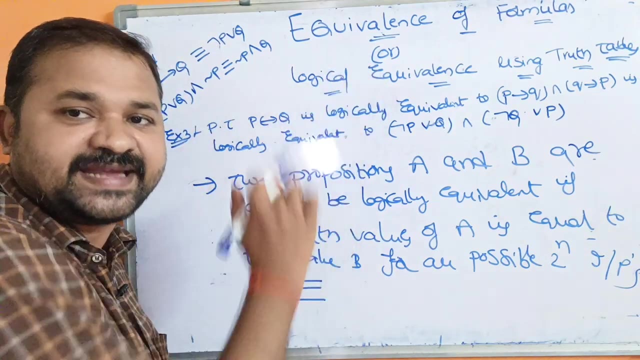 table of A and B are equivalent. Now let us see how we can denote this equivalent. We can denote the equivalent using two symbols. The first symbol is using three horizontal lines. So by using these three horizontal lines, we can represent equivalent, or we can use biconditional operator. 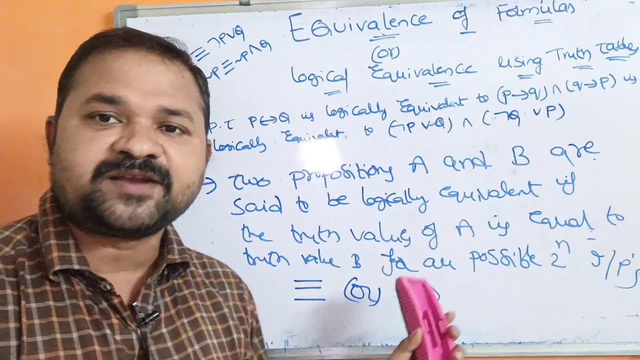 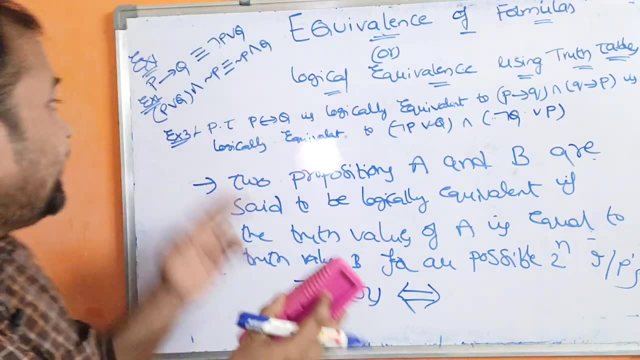 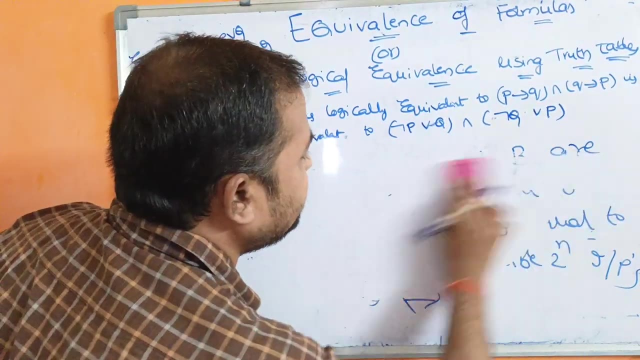 So two horizontal lines, left angular bracket, right angular bracket, So we can use these two symbols in order to represent equivalent. Now let us solve these three examples. So we have to determine whether these two, these three problems, whether they are logically 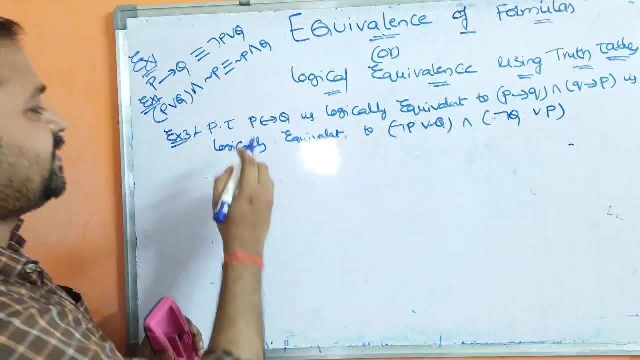 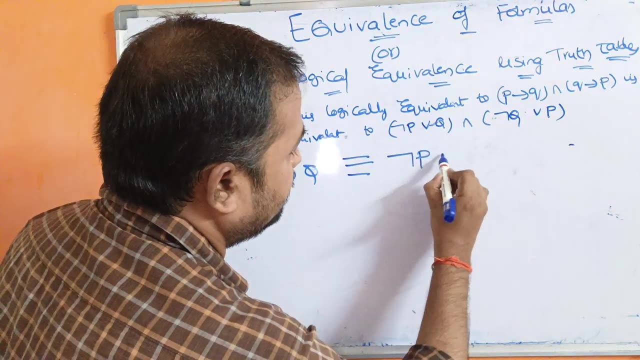 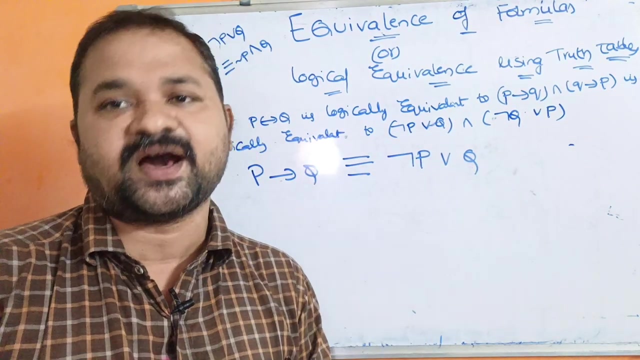 equivalent or not. Let us see the first problem, Example 1.. P implies Q logically equivalent to negation PRQ. So we have to, we have to show that P implies Q proposition is logically equivalent to negation PRQ. So this symbol is called as what: 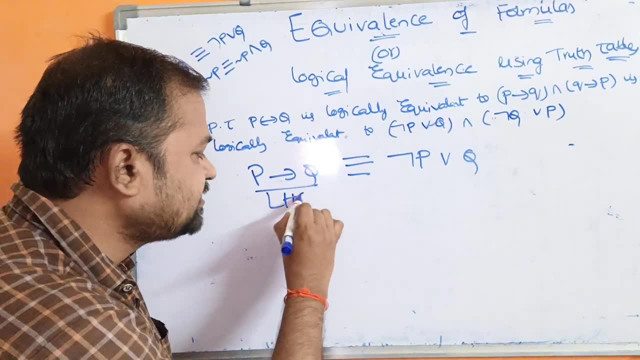 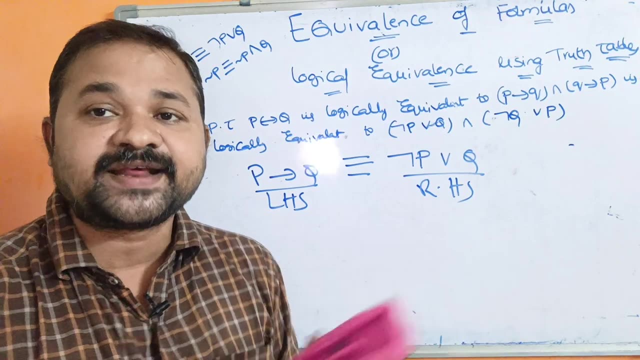 Equivalent symbol. So this is nothing but LHS, This is nothing but RHS. After calculating the truth table, if LHS column is same as the RHS column, then we can say that those function are equivalent. But if we calculate LHS column is same as the RHS column, then we can say that those function are equivalent. For example, if we calculate S bar equal to S, bar equal to 1.、گ and S is equal to 0.. Thank you. 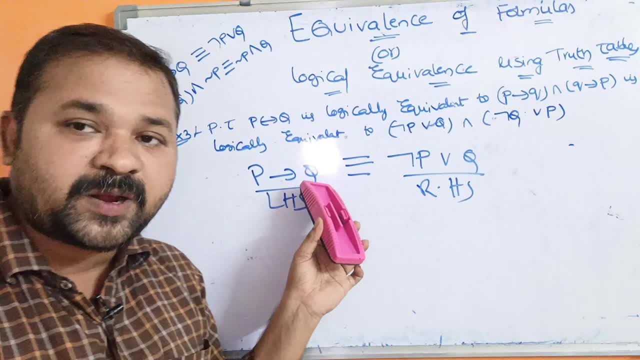 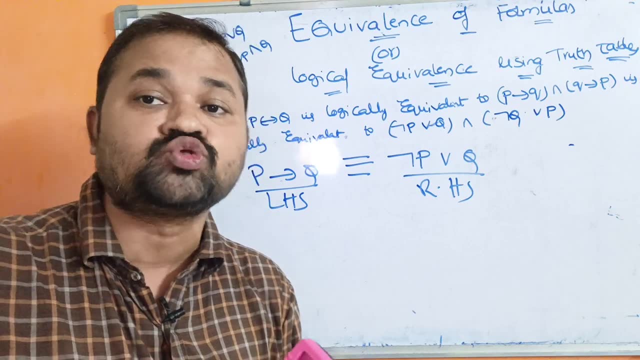 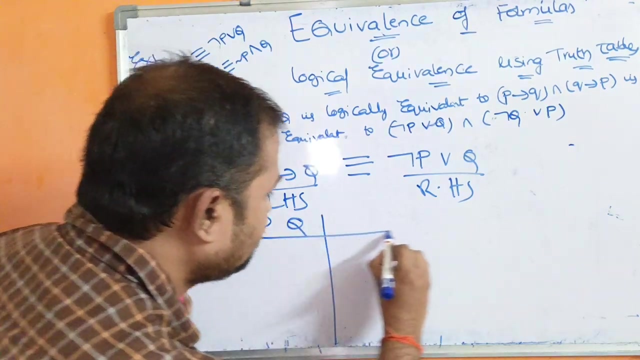 two propositions are logically equivalent Here. how many propositions are there? We have only two propositions, p and q. So the number of possible inputs are 2 power n, that is 2.. 2 power 2 means what? 4.. So four possible combinations are possible. So pq. So next we have to calculate. 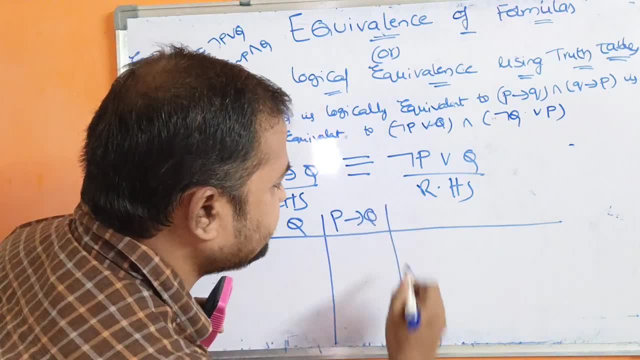 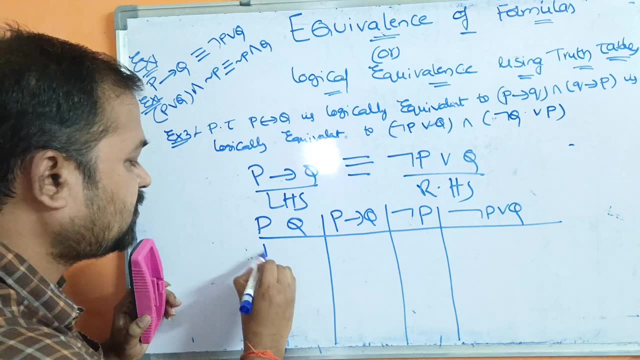 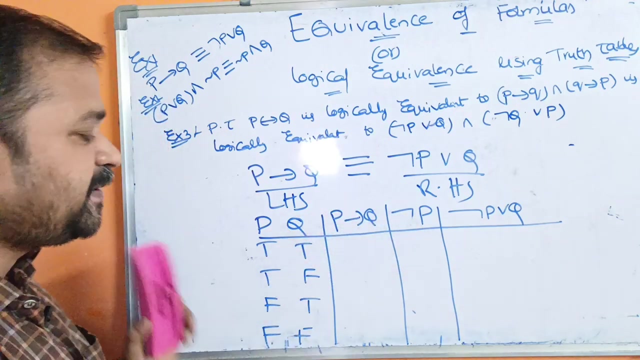 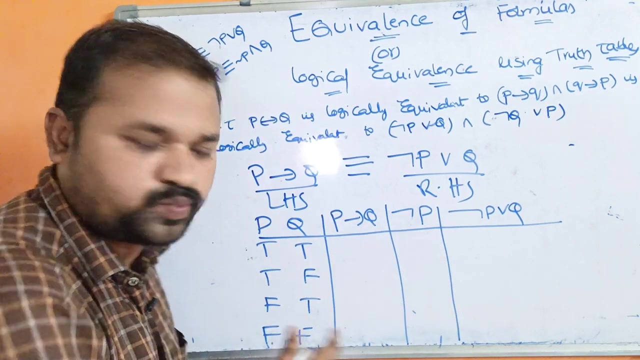 p implies q. Next, let us calculate negation p. Next to calculate negation prq: Negation prq. So the possible values are: true, true, true, false, false, true, false, false. So what is? p implies q. When both propositions are true and false, then the result is false. Otherwise, the result is true. 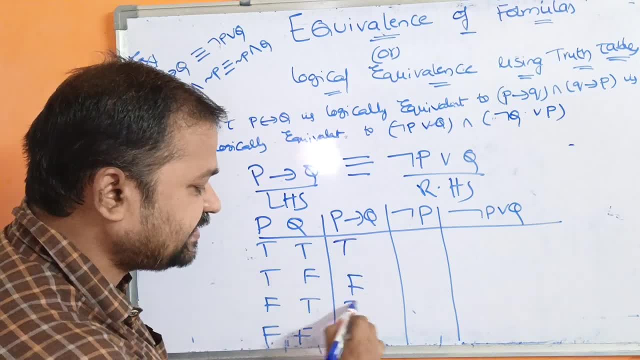 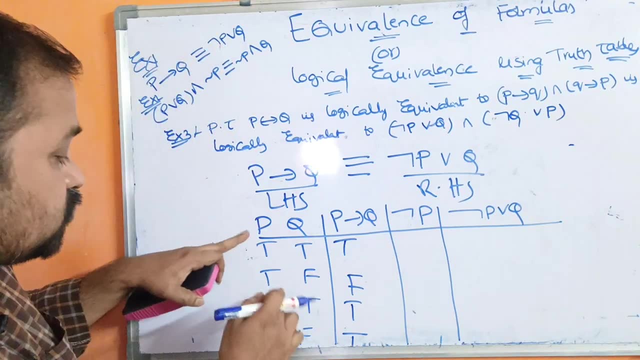 So true, false means false. In remaining three cases, the result is true only. Next we need to calculate negation p. Negation p means what We have to invert b. So true, true, True is inverted to false. True means false. 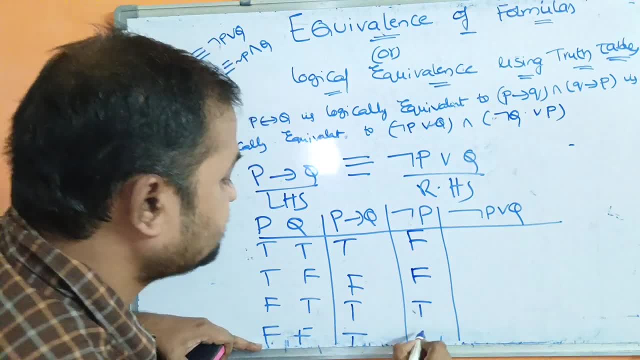 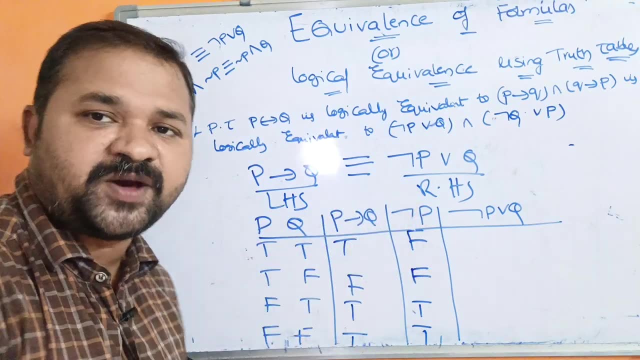 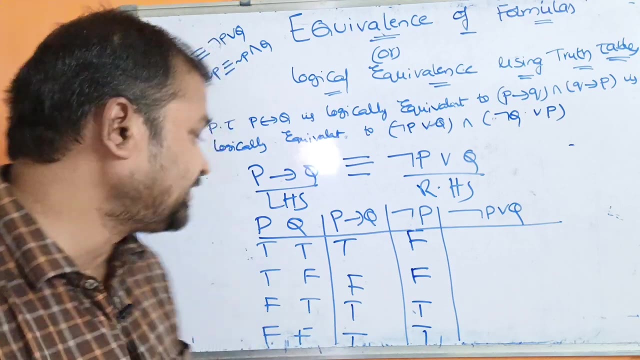 False. So false means true, False means true. Next, we have to calculate negation p, rq. So second column. and on the fourth column we need to perform r operation. We know what is r. When both propositions are false, the result is false. Otherwise, the result is true. So true, false means. 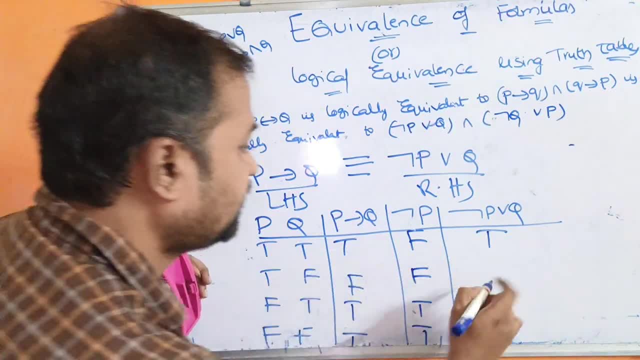 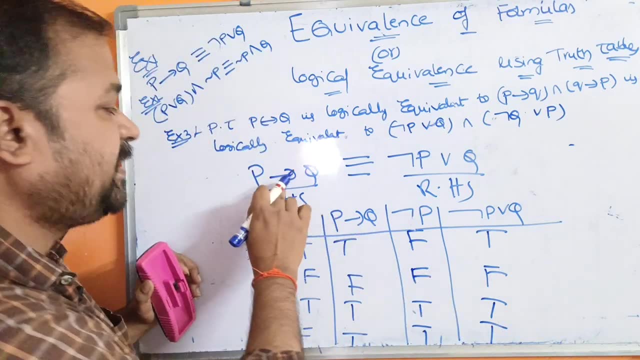 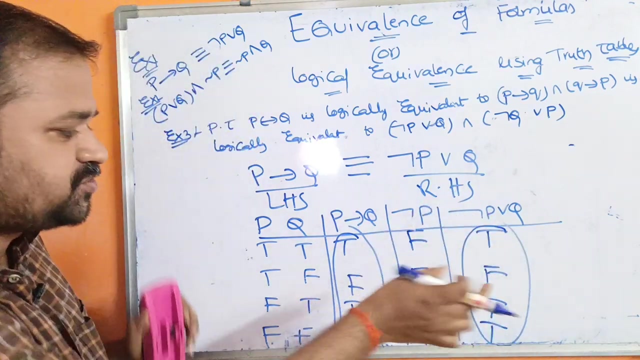 true, False, false means false, True, true means true, False, true means true. p implies q. So this is the left hand side. Negation p: rq. This is the right hand side If we observe these two columns: True, false, true, true, True, false, true, true. So here, left hand. 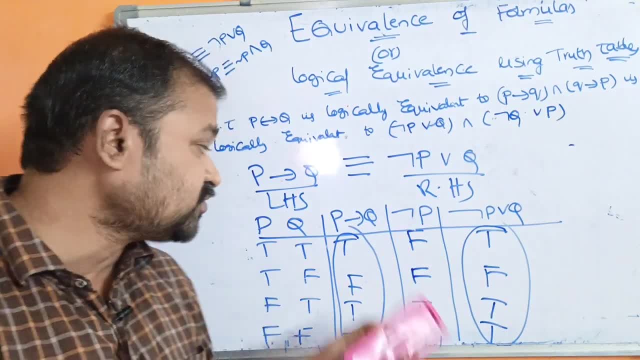 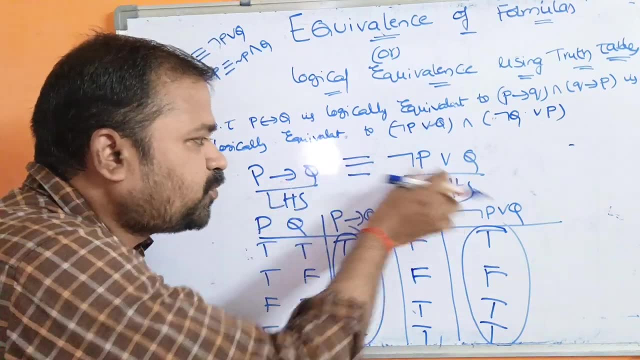 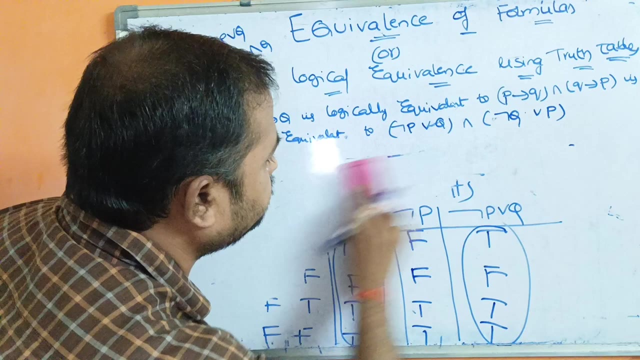 side is equal to the right hand side. Why? Because the truth values of the left hand side is equal to the truth value of the right hand side. So we can say that these two propositions are logically equivalent. Let us solve the second problem. Let us solve the second problem. So what is the second? 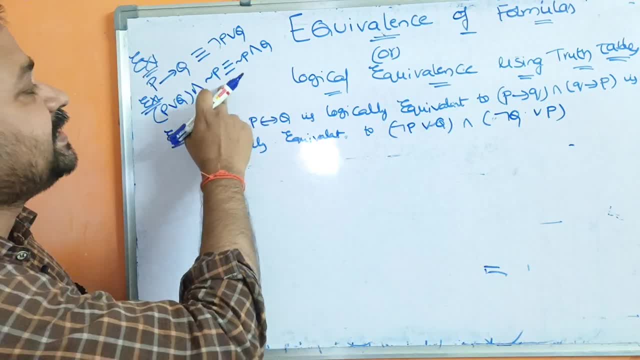 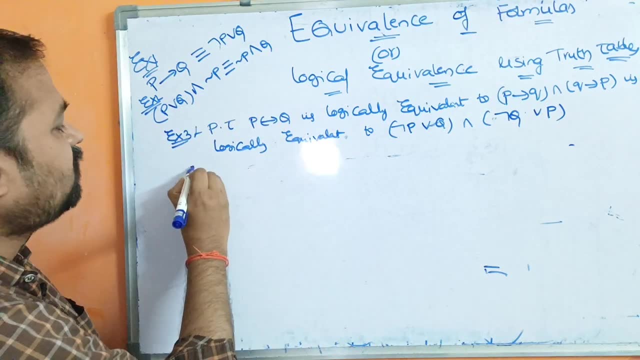 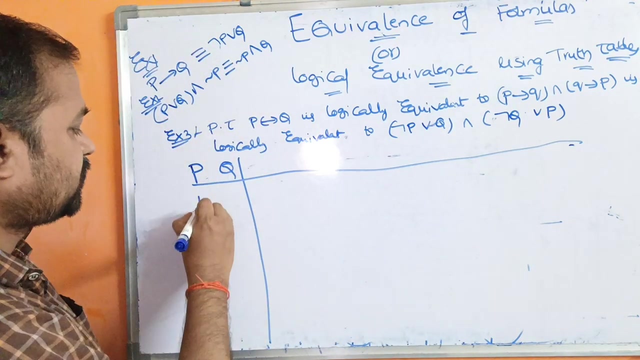 problem p, rq and negation p logically equivalent to negation p under q. So first here we have only two propositions, are there? So the possible combinations are: 2, power, 2. So that is nothing but 4.. So the possible combinations are: true, true, true, false, false, true and false, false. 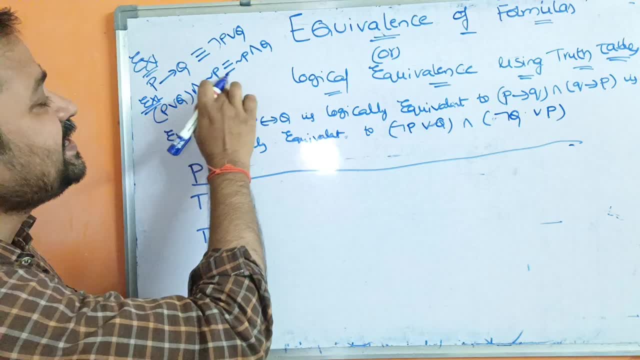 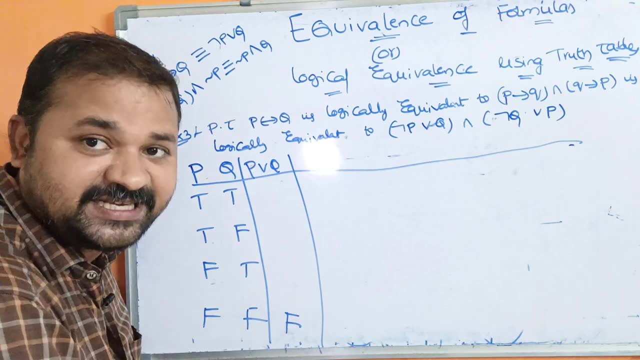 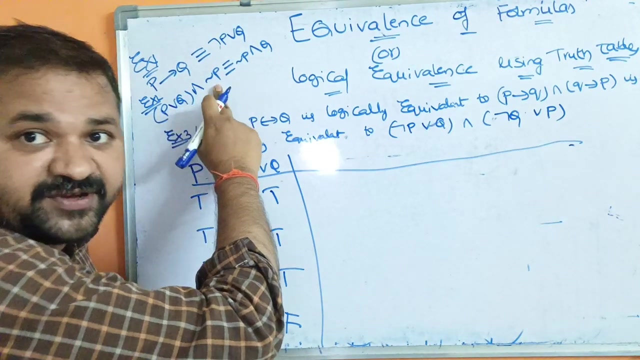 So what is the left hand side? p? rq and negation p. So first we calculate p rq. So what is p? rq? If both propositions are false, the result is false. Otherwise the result is true. Next we have to perform under operation on these two. So we need to calculate negation p. So how to calculate? 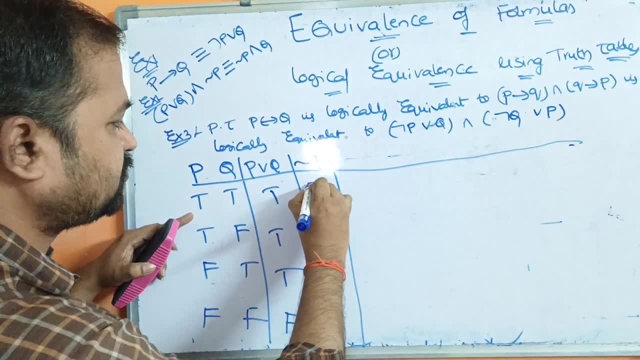 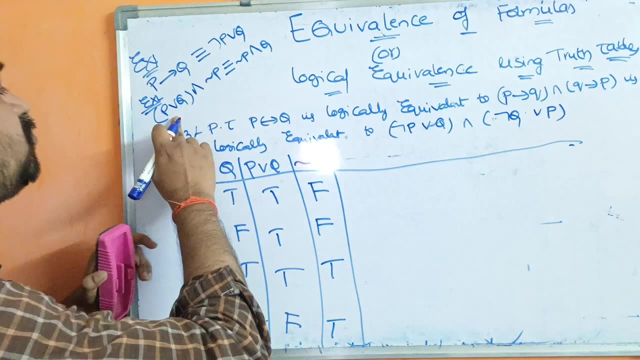 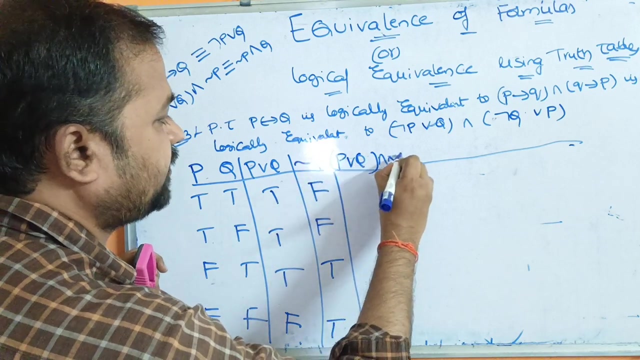 negation p, So negate p values. True means false, True means false, False means true, False means true. Next, we have to perform under operation. Under operation on p, rq and negation p, So we need to perform under operation. So what is? and when both propositions are true, the result is true. 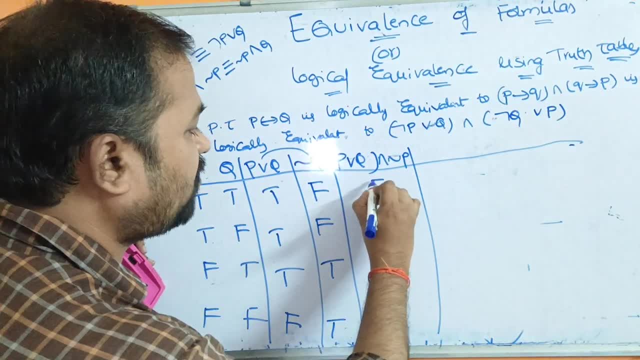 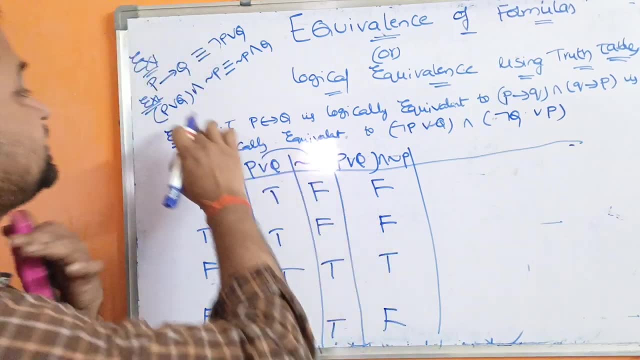 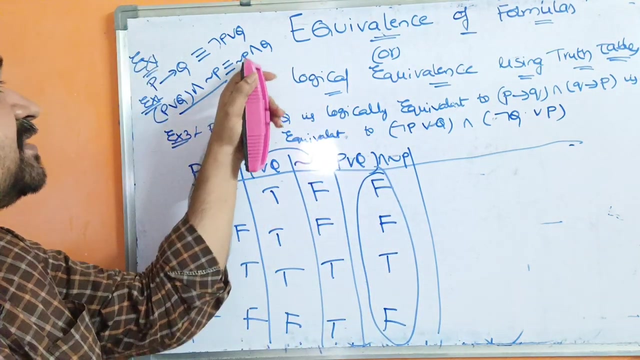 Otherwise the result is false. So true- false means false. True- false means false. True. true means true. False, true means false. So this is nothing but LHS. So this is nothing but LHS. So LHS is calculated. Now we have to determine the RHS. What is RHS? Negation p and q: Negation p and q: 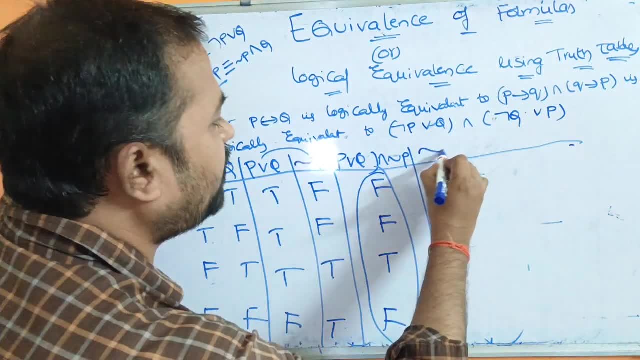 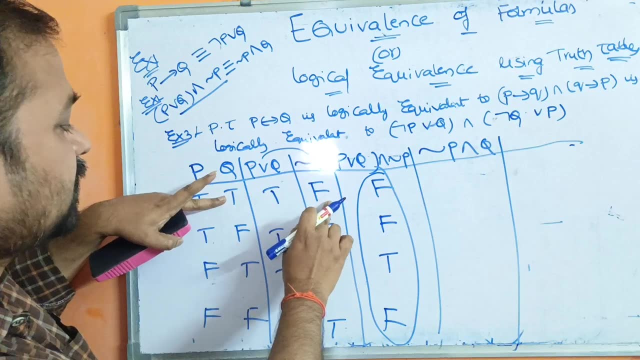 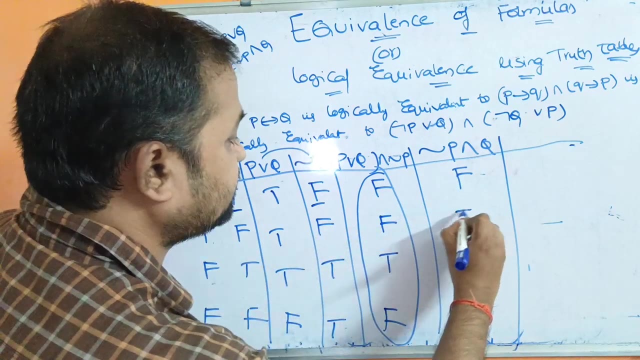 So already negation p is calculated. Next we have to perform under operation with the q. So what second column and fourth column? On second and fourth column, perform the under operation. True, false means false, False, false means false, True, true means. 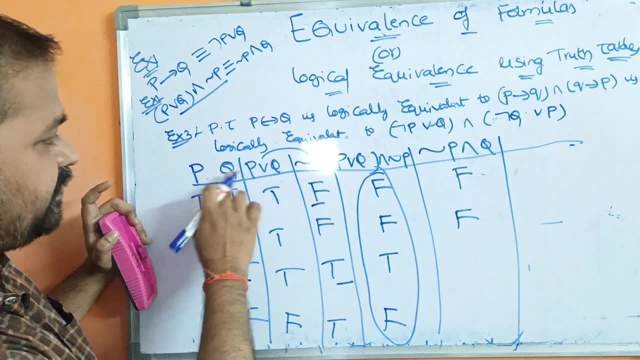 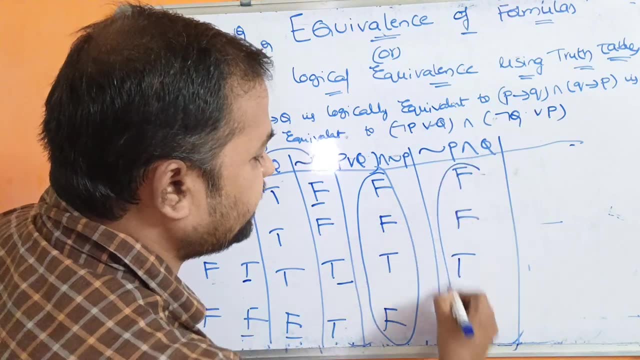 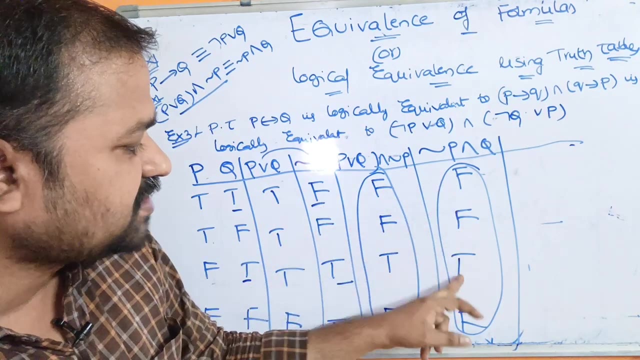 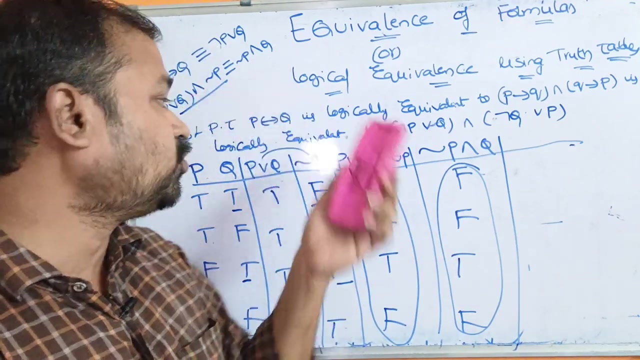 true, False, false means false, So this is nothing but RHS. So if we observe the third column, LHS and the RHS- False, false, true, false, False, false, true, false- So we can say that this problem is also logically equivalent. These two propositions are logically equivalent. Okay, Now let us solve the 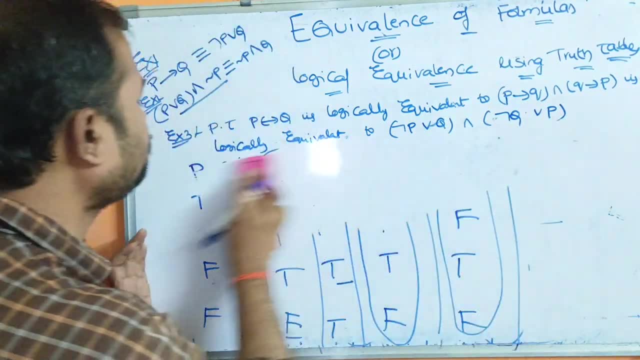 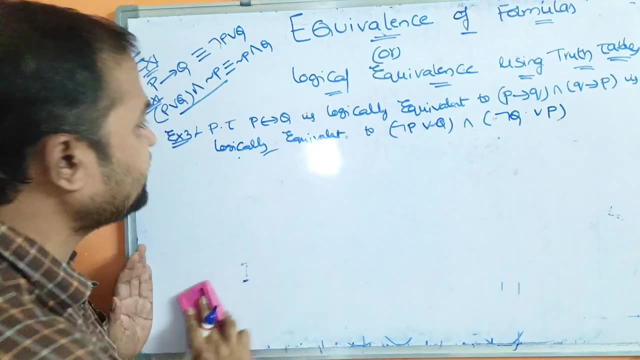 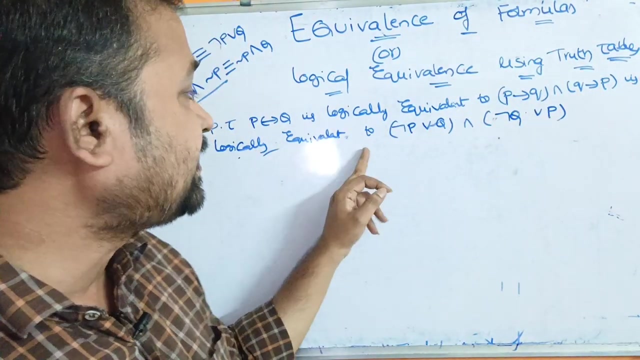 last problem: Prove that. So we have to prove that p biconditional q, p biconditional q, p biconditional q is logically equivalent to p implies q and q implies p is logically equivalent to negation p or q. and 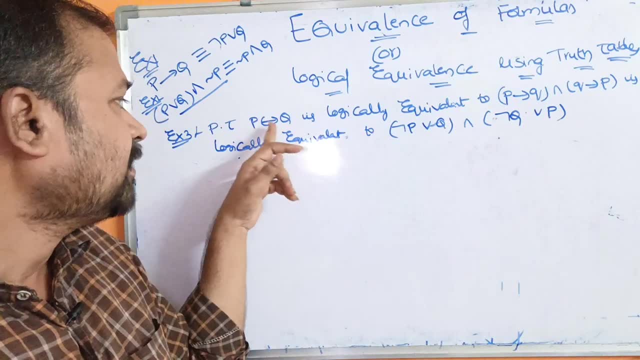 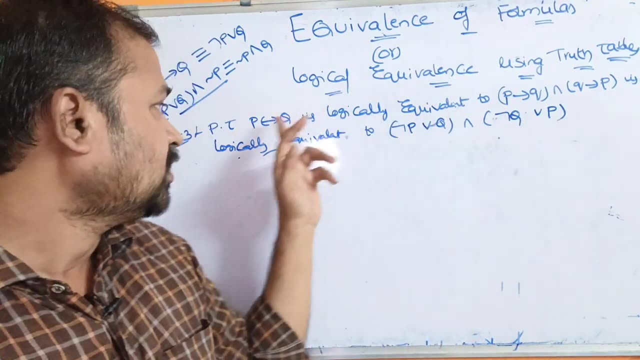 negation q or negation p. So we have to prove that p implies q is similar to this truth table as well, as this is also similar to this table. Okay, So p implies p, double implies q. as well as this proposition and this proposition need to produce 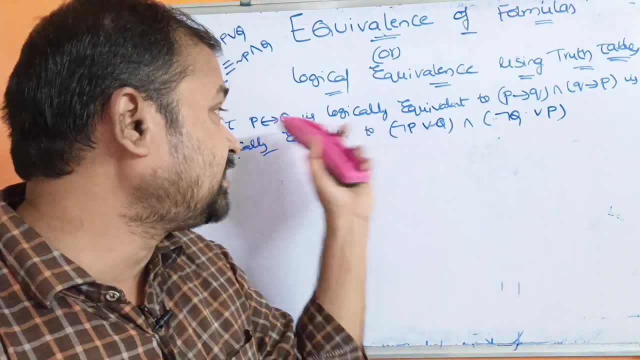 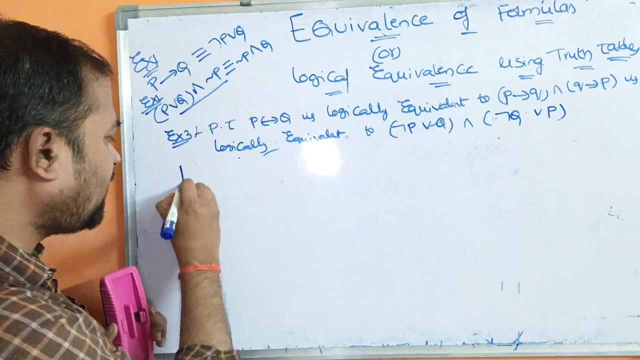 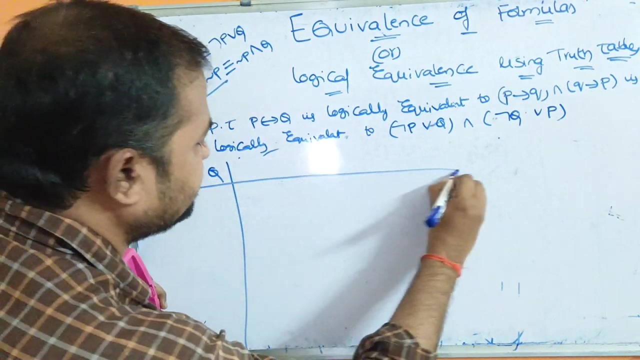 all the values. So if, if these three propositions produces same value, then we can say that those three are logically equivalent. Okay, So here we have only two propositions, are there? So then the possible combinations are: two power, two combinations. So true, true, true, false, false, true. 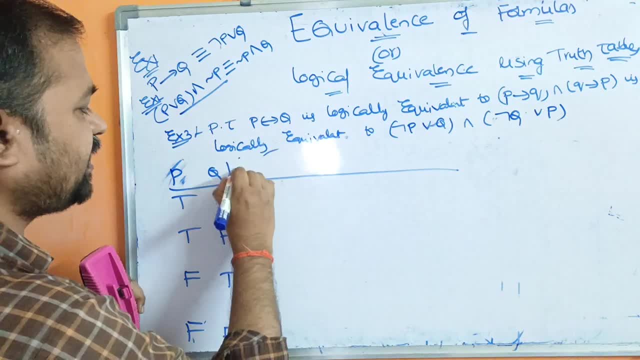 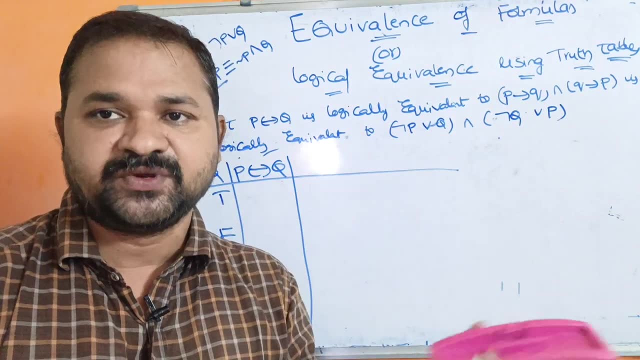 false, false. So first to calculate b biconditional q. So we know what is biconditional. If both propositions contain same truth value, then the result is true. Otherwise the result is false. So true, true, same value. So 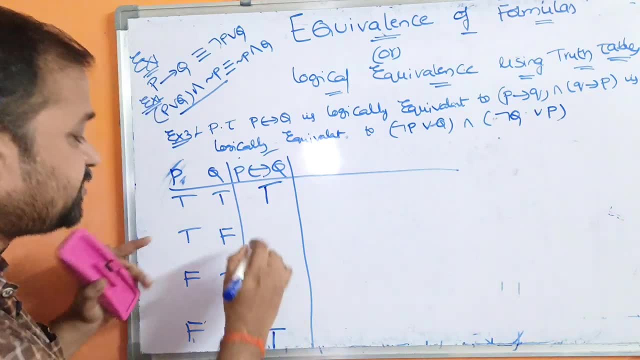 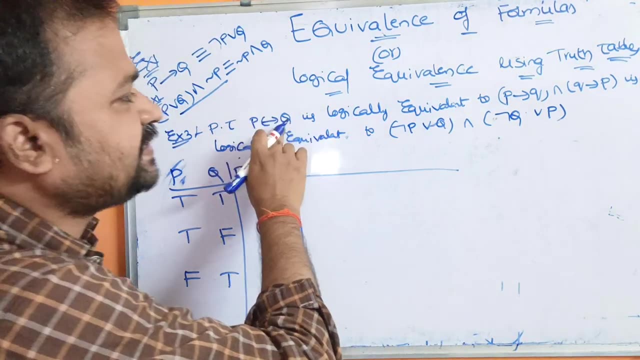 the result is: true, False, false, same value. So the result is: true, True, false, different values, false, false, true, different values, false. Okay, We have to prove that this is logically equivalent to: p implies q and q implies p. So first let us calculate the value of the result. So, true, true, 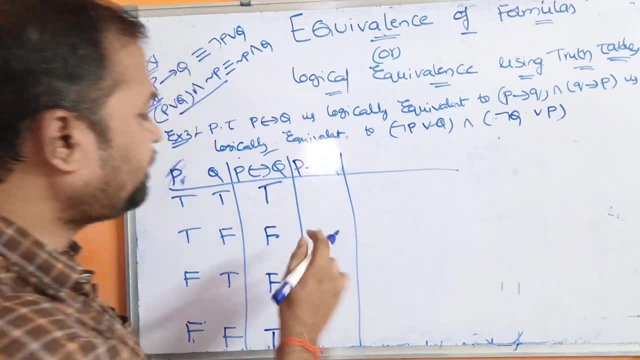 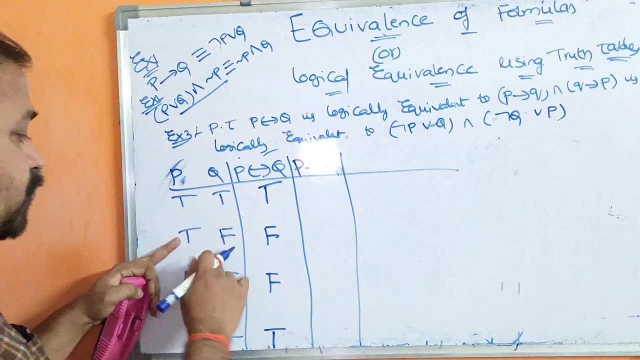 true, false equals to true. Next, to calculate: p implies q equals to true, So p implies can be written as simple: as p implies q, So p implies means what: if both propositions are true, false, the result is false. Otherwise, the result is true, So true, false means false. true true, true, false. 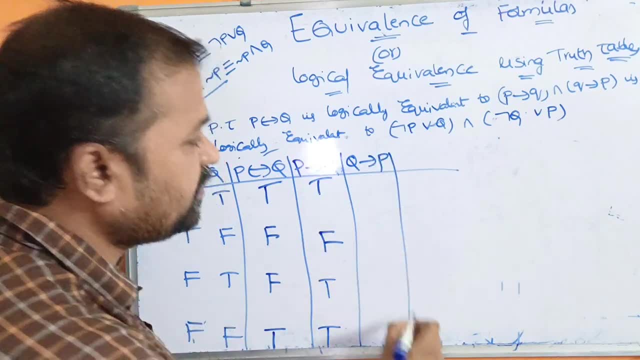 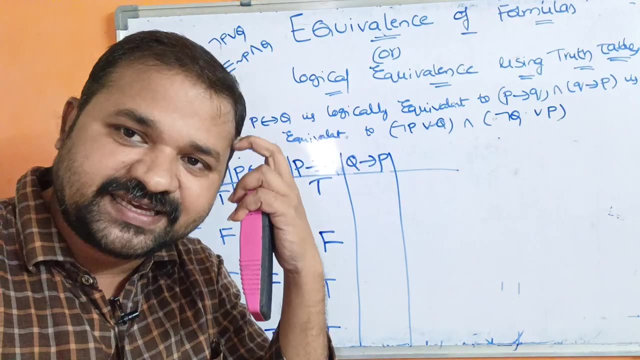 true, true, false, false, true. Next, to calculate: q implies p, Q implies p. So if q is, if q is true and p is false, the result is false. In the remaining three cases, the result is true. 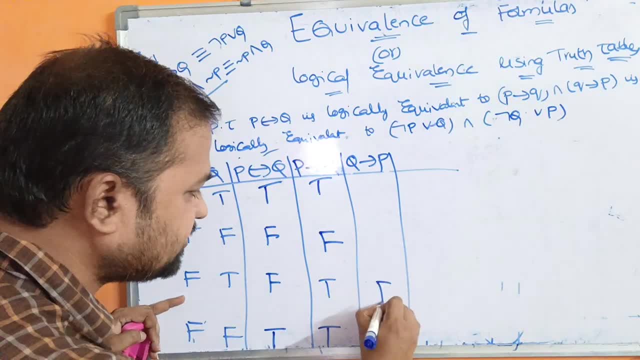 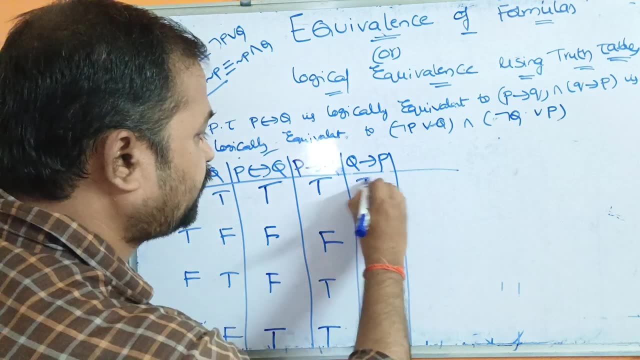 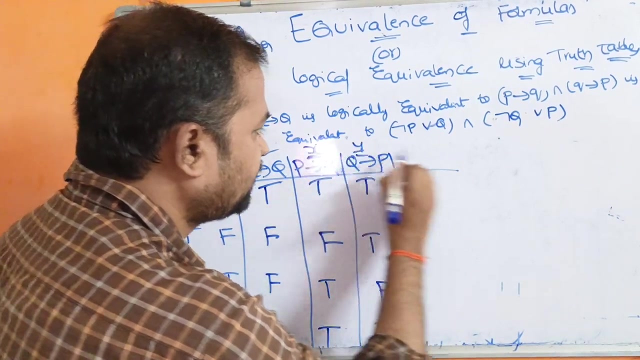 here the q is true, p is false, so the result is false. in remaining three cases: true. true means true, false, true means true, false, false means true. so true, true, true. okay, next we have to perform the under operation. let us assume that this is x, this is y, so we need to perform under operation x and y. 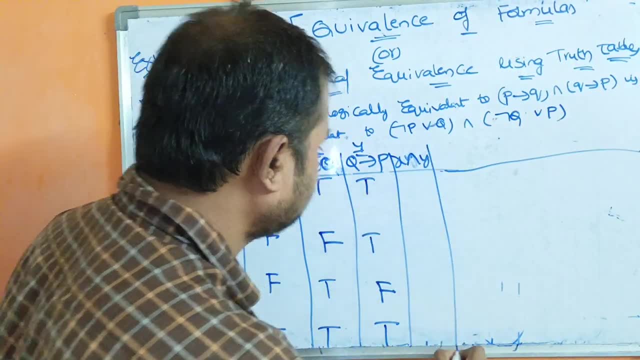 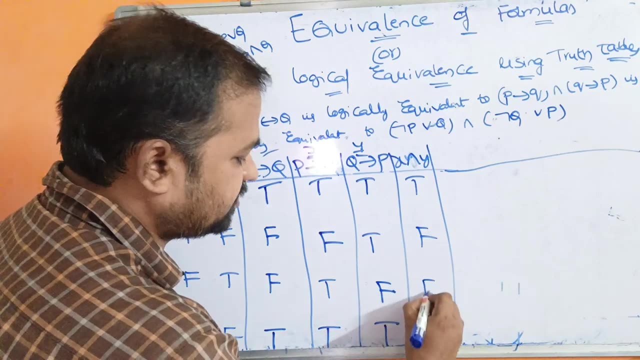 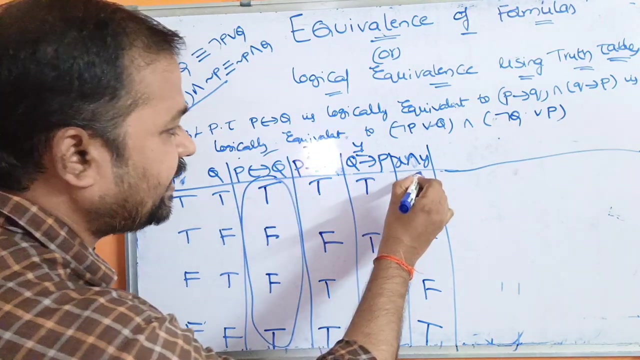 x and y, x and y. so we have to perform under operation. true true means true, false true means false. true, false means false. true, true means what is true. true, true, true means true. if we observe p by conditional q column and p implies q and q implies p, what is the result? true. 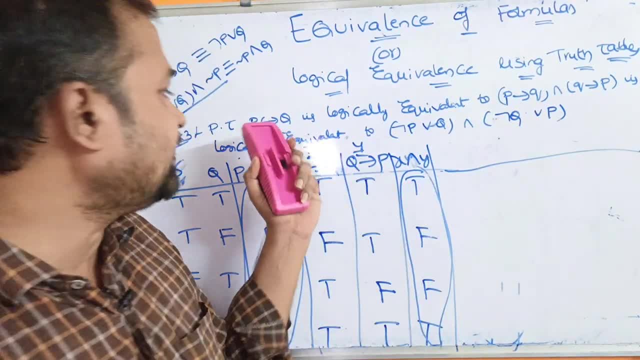 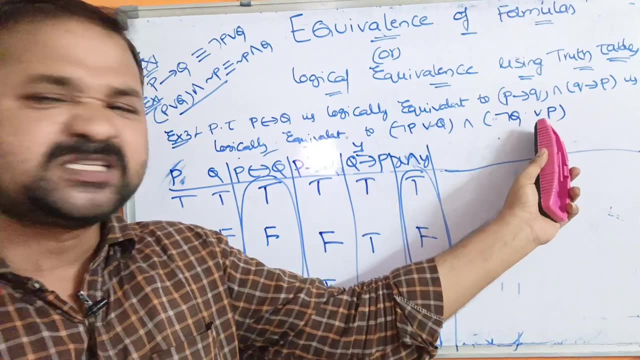 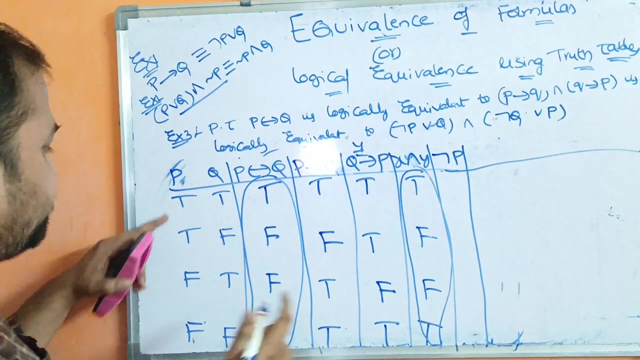 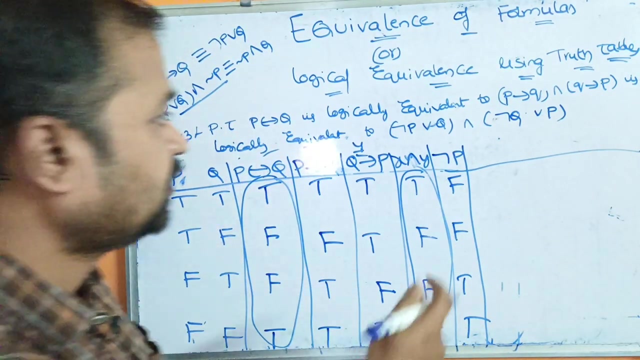 false, false, true, true, false, false, true. so we can say that these two prepositions are logically equivalent. now we have to prove that this preposition is logically equivalent to this preposition, so here we need to compute negation p. so what is negation p? true, true, false, false, so false, false, true, true, true, true, false, false, so false, false, true, true. 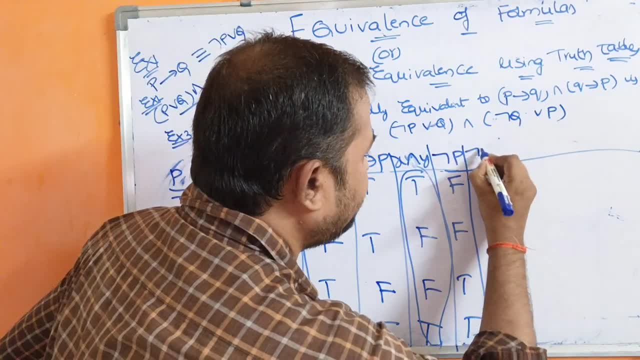 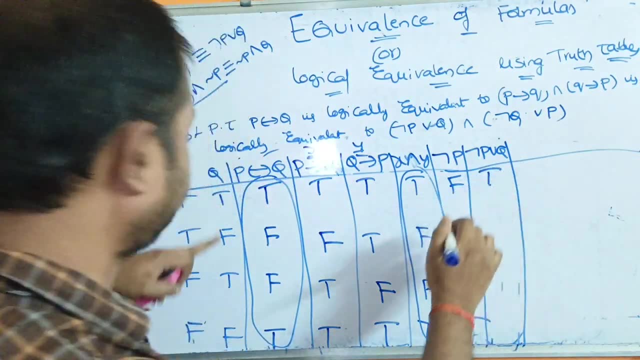 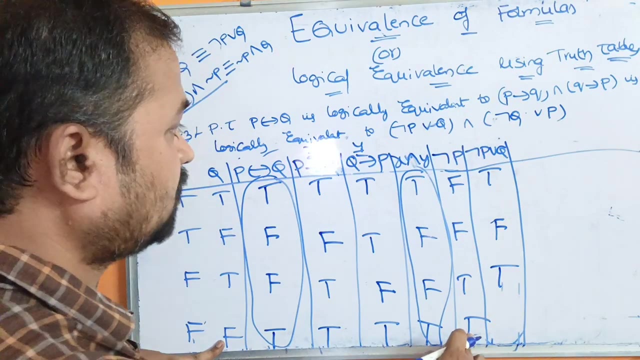 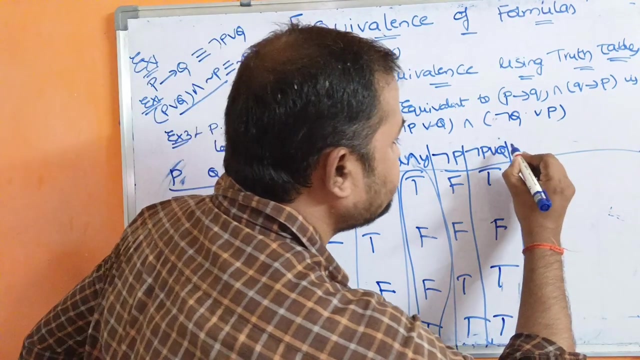 so already we have q is there. so let us calculate this one: negation p or q. here we have negation p, here we have q. so true, false means true, false, false means false, false, true, true means true, false, true means true, false, true means true. okay, so negation p or q is over. next we need to calculate negation q.